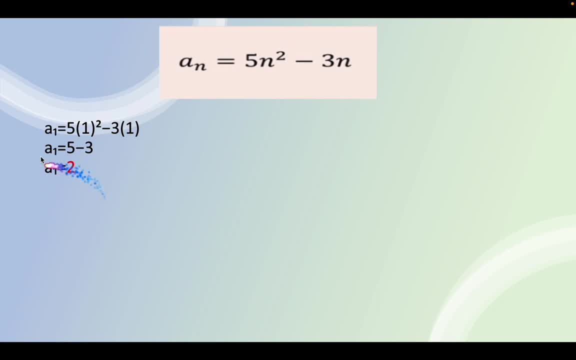 So for the first answer, for the first term will be number 2.. So next Next term is for second term. So a sub 2 equals 5 times 2, squared minus 3 times 2 is a substitute lampu young, second term and since second. 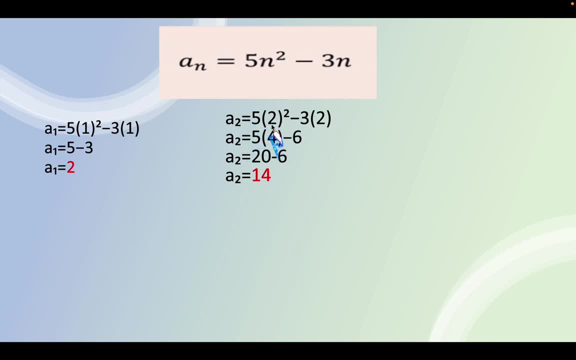 napusha. so the number that we'll use is number 2. so 5 times 2 squared minus 3 times 2, and then a sub 2 equals 5 times 4, since 2 squared is 4, and then minus 6, since 3 times 2 is 6, and then a sub 2 equals 20 minus six, five times four. 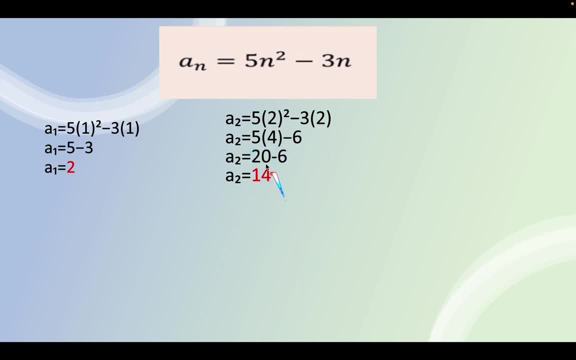 is 20 minus six. so the answer for the second term is 14. third term: for the third term, a sub 3 equals 5 times 3 squared minus 3 times 3, And then a sub g equals 5, since g squared is 9 minus g times g is 9.. 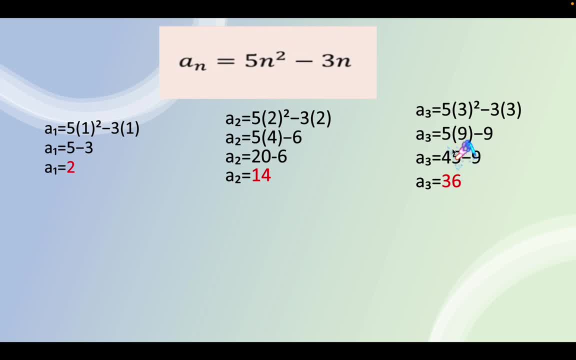 So for the answer is: 5 times 9 is 45.. Then copy minus 9.. So for the answer for the third term is 36.. Okay, Next for fourth term. For fourth term, the answer will be: a sub 4 equals 5 times 4 squared minus g times 4.. 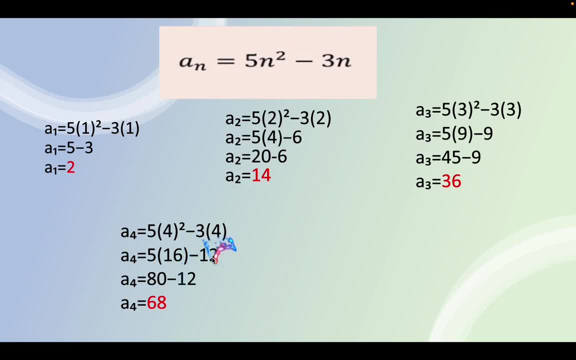 4 squared is 16, and then g times 4 is 12.. Then a sub 4 equals 80, since 5 times 16 is 80.. Copy minus 12.. So the answer for the fourth term is, And for the last term it will be: a sub 5 equals 5 times 5 squared minus g times 5..